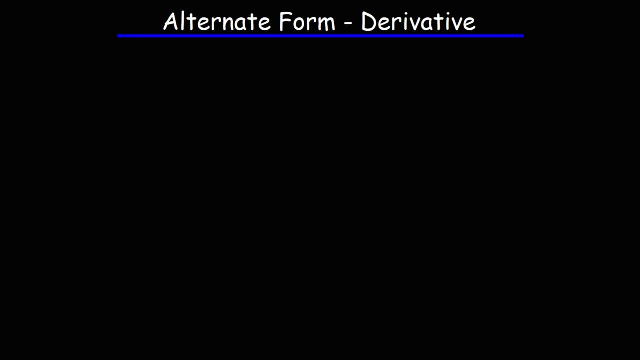 Let's talk about the alternative form of the derivative. Now let's say we have some function f of x and let's define it to be equal to x cubed. Now we know what the first derivative of that function is. Using the power rule, the derivative of x cubed is going to be 3x squared. 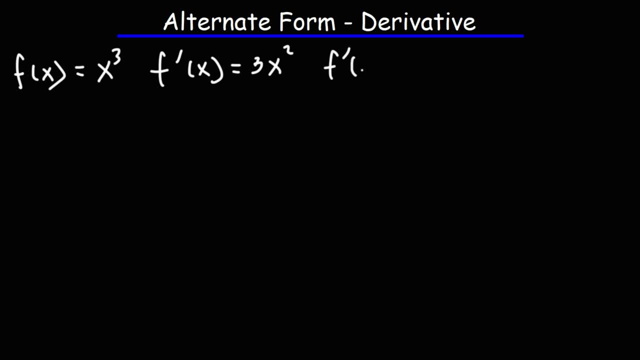 Now let's say, if we plug in some point, let's say 4.. This is going to be 3 times 4 squared, which is 3 times 16, that's 48.. So this is the derivative of f, of x as a function and this number. when we evaluate the derivative, 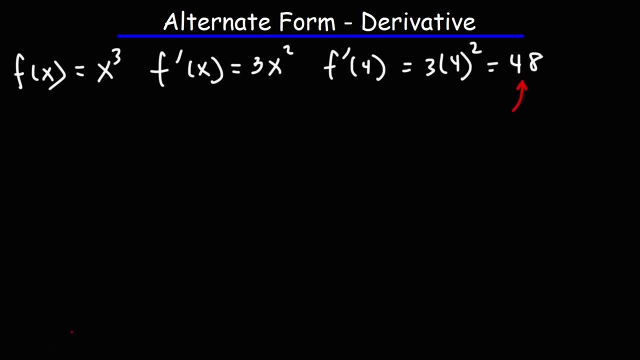 at a point we get the slope of the tangent line. Now we can find the derivative of the function using limits. So f prime of x is equal to the limit as h approaches 0 of f of x plus h minus f of x divided by h. 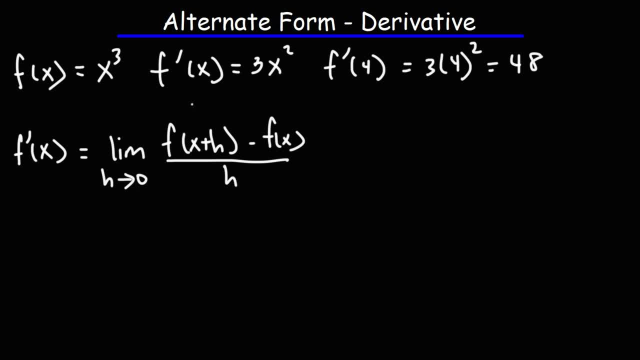 So this is the limit definition of the derivative and using this formula it will give us: f prime of x is equal to 3x squared. Now the alternative form of the definition of the derivative is this equation: f prime of a is equal to the limit as x approaches a, of f, of x minus f, of a over x minus a. 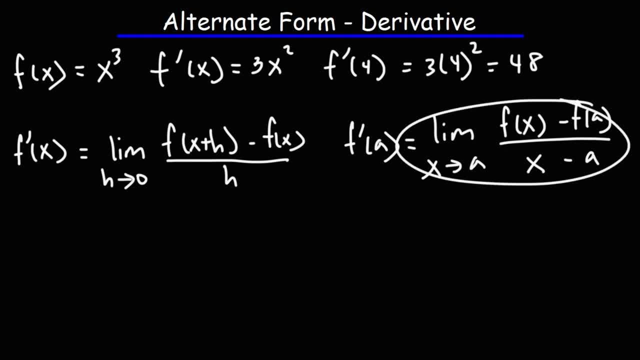 Now this form of the derivative. it will give you a number, as opposed to a function that depends on x. So using this, you can get the slope of the tangent line, which is 48 when x is 4.. So make sure you understand the difference between these two formulas. 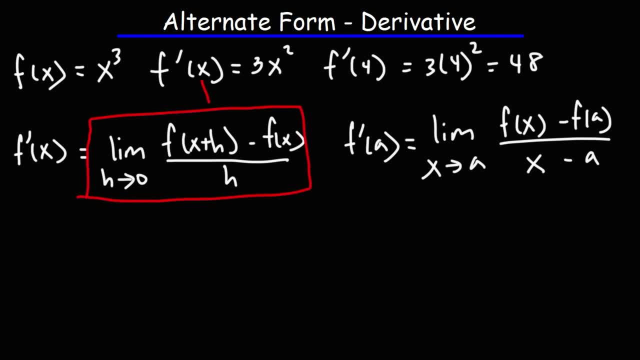 So this formula will give you the derivative as a function and this formula will evaluate that derivative at some point where x equals a. Let's use both of these two formulas So you can see how it works. So let's start with this one. 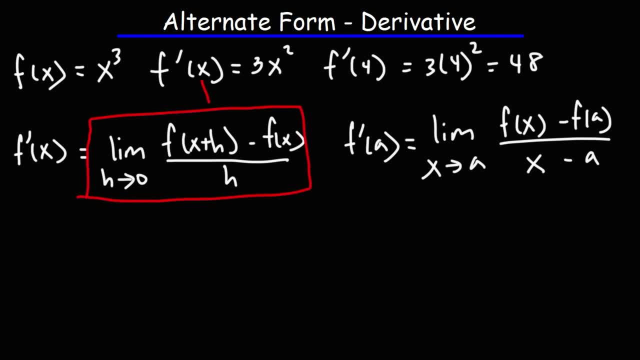 So this formula will give you the derivative as a function and this formula will evaluate that derivative at some point where x equals a. Let's use both of these two formulas So you can see how it works. So let's start with this one. 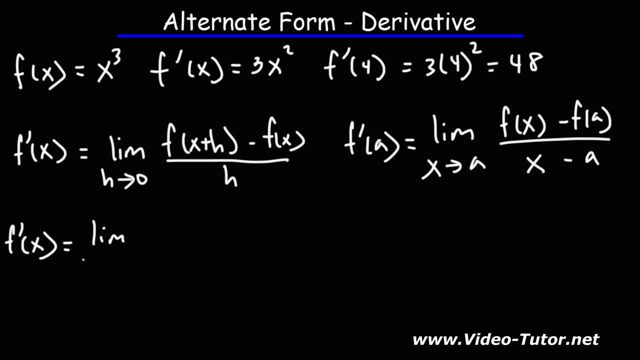 So f prime of x is going to be the limit as h approaches 0, and then we have f of x plus h. So in this formula we're going to replace x with x plus h, So x cubed will become x plus h cubed. 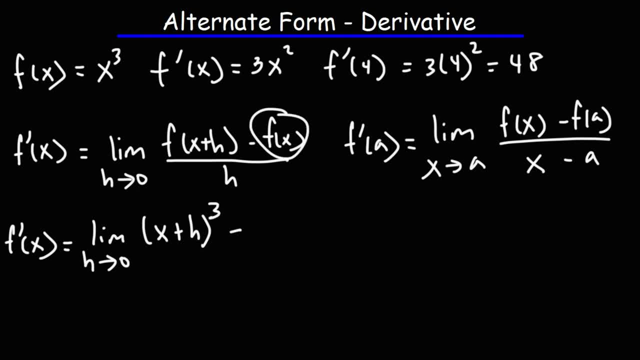 Now minus f of x. so f of x is simply x cubed and then divided by h. So now, how can we evaluate this limit? Notice that we have a difference of two cubes When you see that we could use this formula. 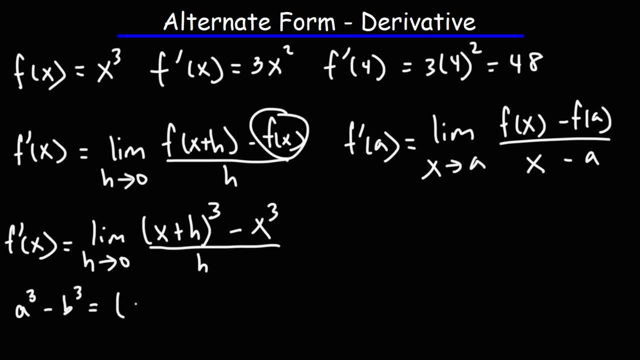 a to the third minus b to the third is going to be a minus b times a squared plus ab plus b. So in that example a is going to be x plus h, b will be x. So a minus b, that's going to be x plus h, that's a, and then minus b minus x. 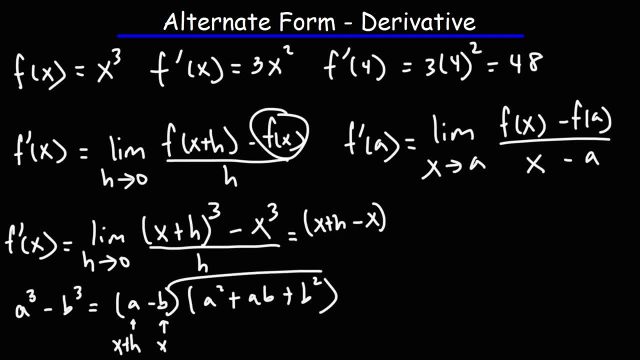 So that part is just the a minus b part. Now we need this part. So a squared, that's going to be x plus h squared, Then a squared, that's going to be x plus h squared, Then a times b. so we're multiplying these two. 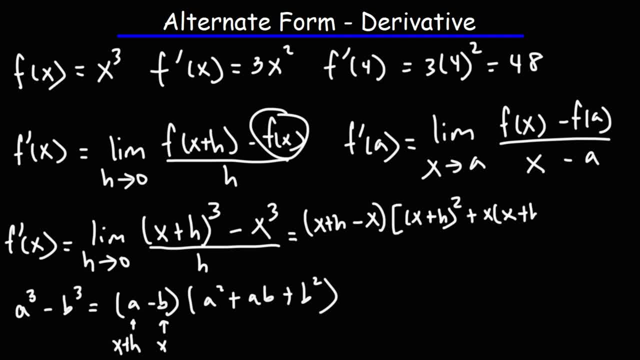 That's going to be x times x plus h, or you can write it in reverse, so it'll be the same. And then, plus b squared, b is x, so b squared is x squared, And this is going to be divided by h. 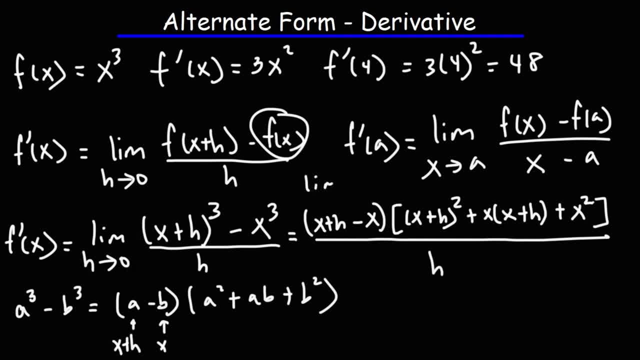 Now, of course, I need to rewrite this expression, So this is as the limit as h approaches zero. Now x and negative x will cancel. So what we have left over is the limit as h approaches zero. We have an h left over, so it's h. and then times x plus h squared plus x. times x plus h. times x squared. 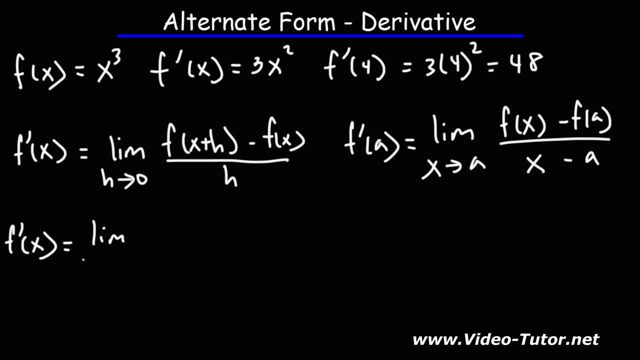 So f prime of x is going to be the limit as h approaches 0, and then we have f of x plus h. So in this formula we're going to replace x with x plus h, So x cubed will become x plus h cubed. 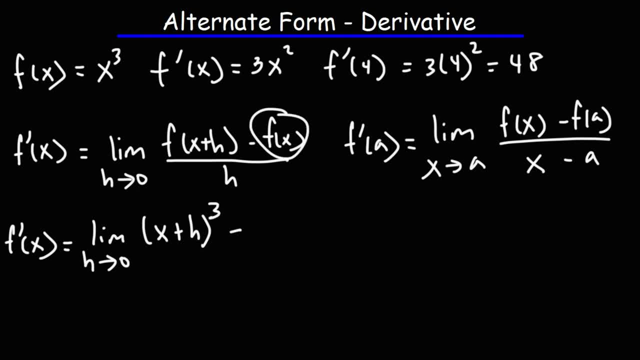 Now minus f of x. so f of x is simply x cubed and then divided by h. So now, how can we evaluate this limit? Notice that we have a difference of two cubes When you see that we could use this formula. 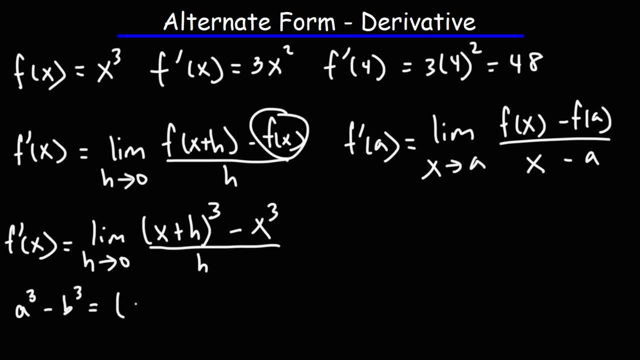 a to the third minus b to the third is going to be a minus b times a squared plus ab plus b. So in that example a is going to be x plus h, b will be x. So a minus b, that's going to be x plus h, that's a, and then minus b minus x. 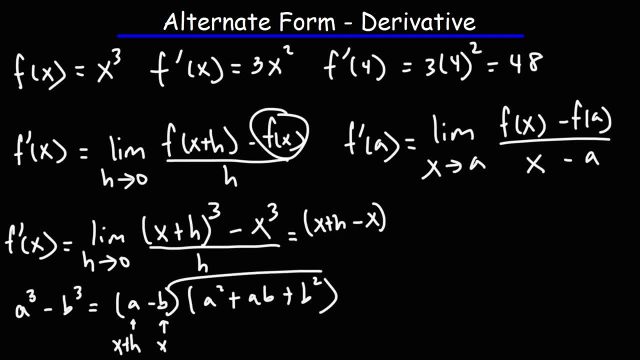 So that part is just the a minus b part. Now we need this part. So a squared, that's going to be x plus h squared, Then a squared, that's going to be x plus h squared, Then a times b. so we're multiplying these two. 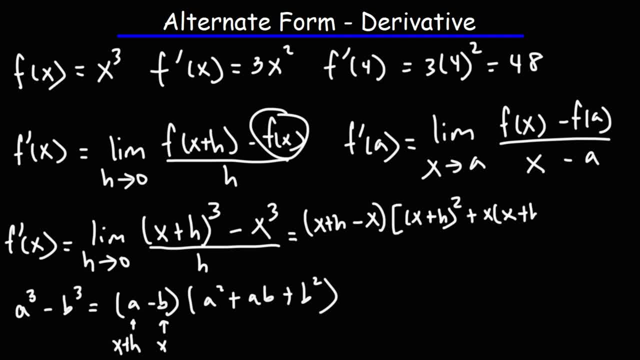 That's going to be x times x plus h, or you can write it in reverse, so it'll be the same. And then, plus b squared, b is x, so b squared is x squared, And this is going to be divided by h. 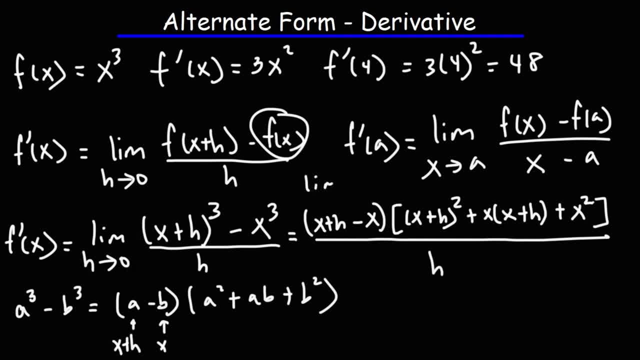 Now, of course, I need to rewrite this expression, So this is as the limit as h approaches zero. Now x and negative x will cancel. So what we have left over is the limit as h approaches zero. We have an h left over, so it's h. and then times x plus h squared plus x. times x plus h. times x squared. 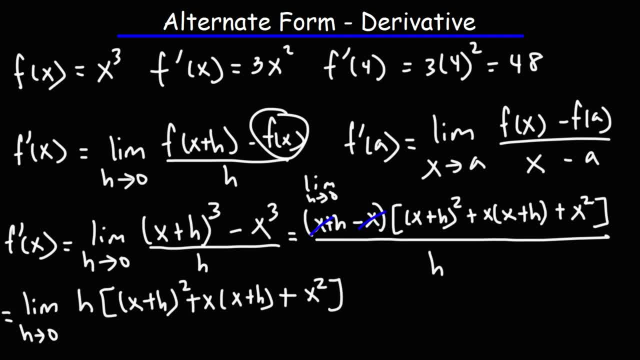 We don't need to FOIL or distribute what we have here. I'm just going to leave it that way. Now notice that we can do this. We can cancel h As soon as the h from the bottom is gone. we can now use direct substitution. 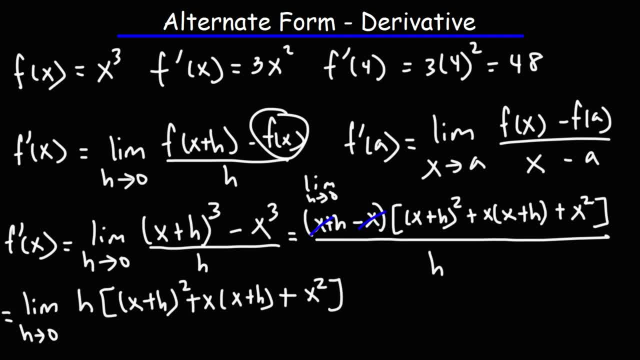 We don't need to FOIL or distribute what we have here. I'm just going to leave it that way. Now notice that we can do this. by doing this, We can cancel h As soon as the h from the bottom is gone. we can now use direct substitution. 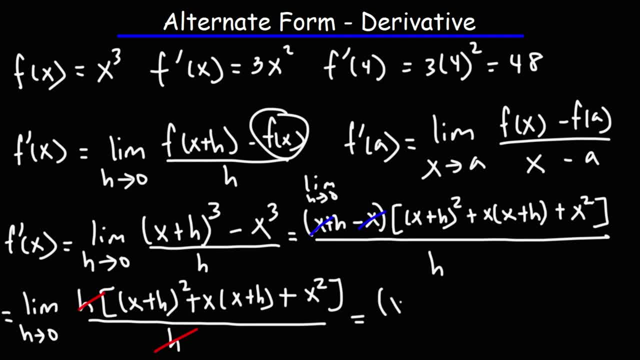 So I'm going to replace the remaining h with zero. So this is going to be x plus zero squared plus x times x plus zero plus x squared. x plus zero squared is just x squared, And then x times x, that's x squared again. 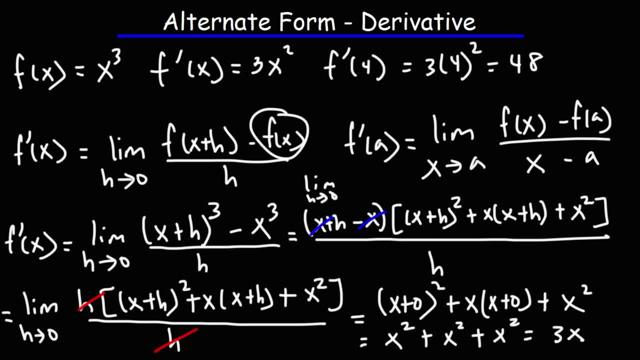 Again, if you add x squared three times, you're going to get 3x squared, And so we can see that these two answers they match. So this formula gives you the derivative as a function. Now let's use the second one. 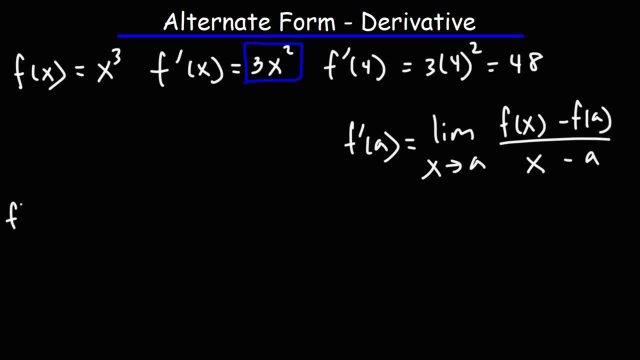 So let's calculate f prime of a. So a is going to be the number inside of f prime, which is four. So we're looking for f prime of four. This is going to be the limit as x approaches four of f of x. 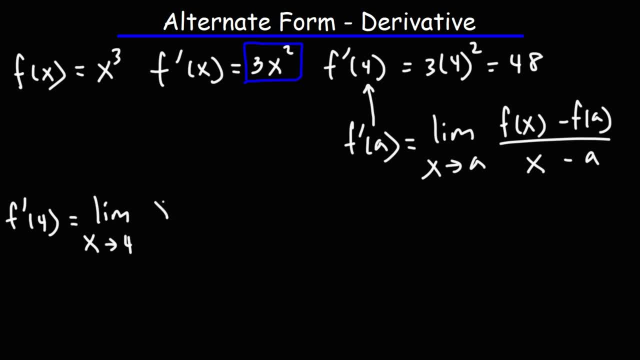 f of x is x cubed minus f of a. So f of a is the same as f of four. So we're plugging four into that function, So f of four is going to be four to the third power, And then over x minus a or x minus four. 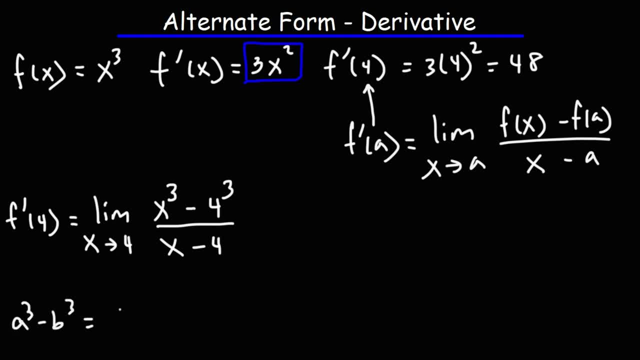 Now, once again, we're going to use the difference of perfect cubes formula, So we're going to factor as a minus b times a squared plus a, b plus b squared, So a is x, b is four. This is going to be the limit as x approaches four. 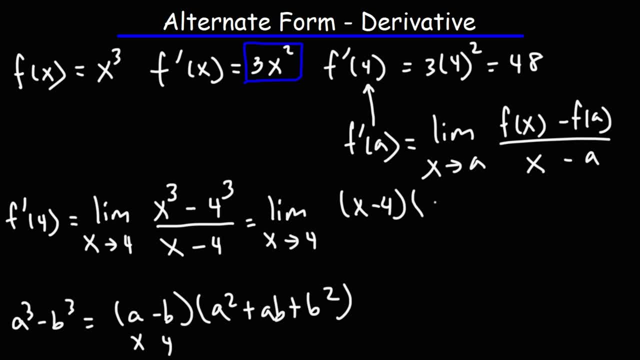 And then. And then x minus four times a squared, that's going to be x squared. And then a times b, that's four times x plus b. squared, b is going to be four squared. And then over x minus four. Now notice that we could cancel x minus four. 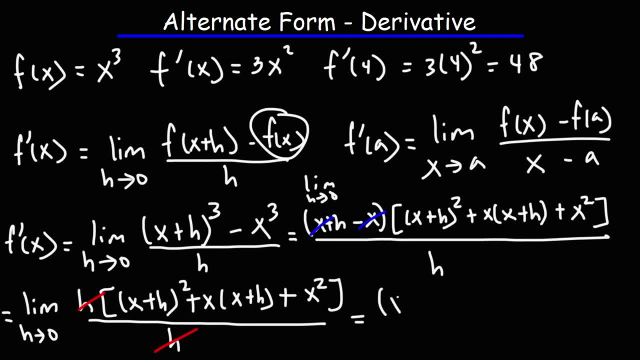 So I'm going to replace the remaining h with zero. So this is going to be x plus zero squared plus x times x plus zero plus x squared. x plus zero squared is just x squared, And then x times x, that's x squared again. 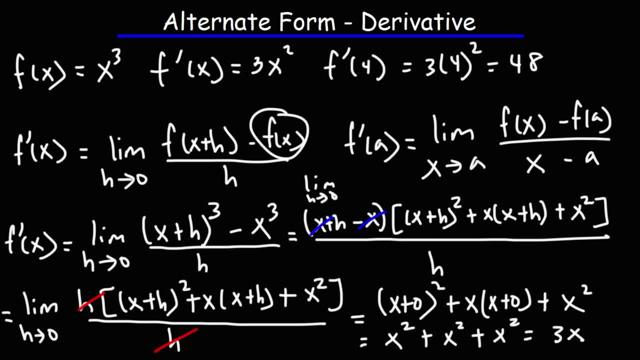 Again, if you add x squared three times, you're going to get 3x squared, And so we can see that these two answers they match. So this formula gives you the derivative as a function. Now let's use the second one. 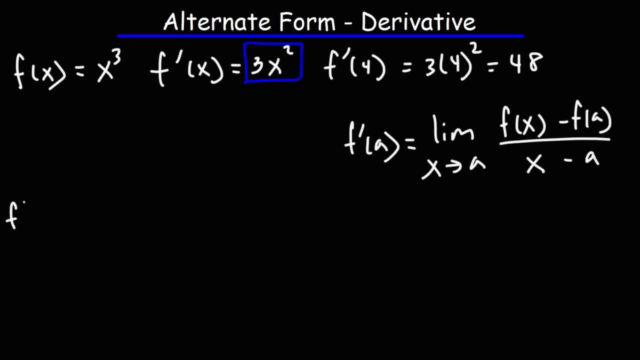 So let's calculate f prime of a. So a is going to be the number inside of f prime, which is four. So we're looking for f prime of four. This is going to be the limit as x approaches four of f of x. 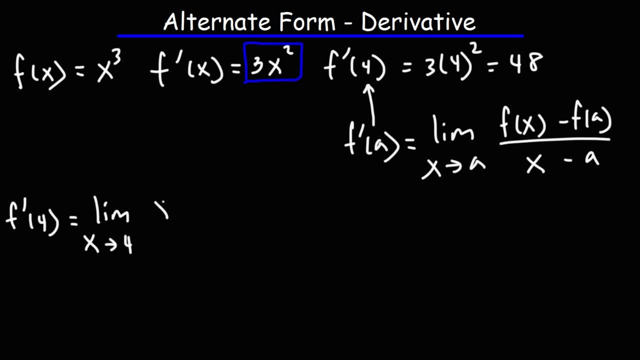 f of x is x cubed minus f of a. So f of a is the same as f of four. So we're plugging four into that function, So f of four is going to be four to the third power, and then over x minus a or x minus four. 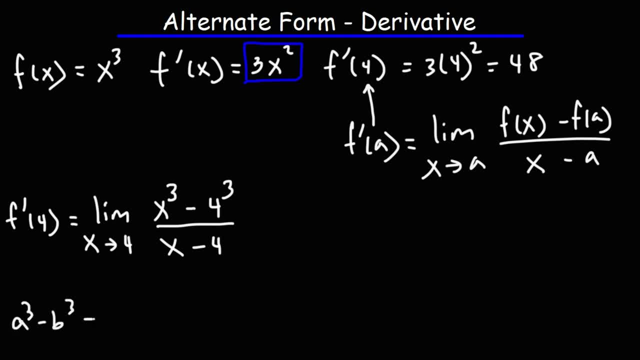 Now, once again, we're going to use the difference of perfect cubes formula, So we're going to factor as a minus b times a squared, plus ab plus b squared, So a is x, b is four. This is going to be the limit as x approaches four. 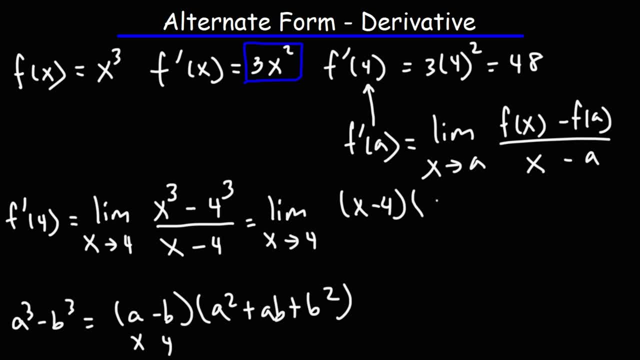 And then x minus four times a squared, That's going to be x squared. And then a times b, That's four times x plus b squared. b is going to be four squared. And then over x minus four. Now notice that we could cancel x minus four. 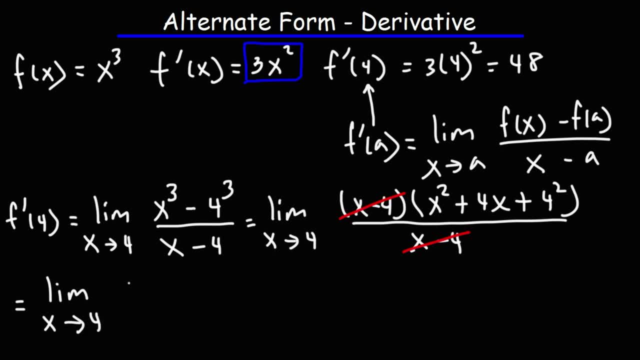 Now, once we do that, we're left with this expression. Now, once we get rid of the x minus four on the bottom, we can now use direct substitution. So replace an x with four. We're going to have four squared plus four times four plus four squared.